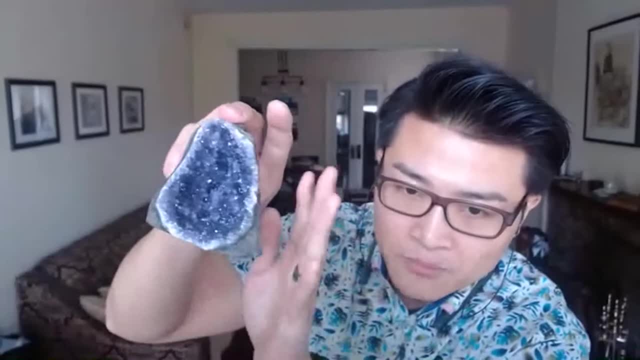 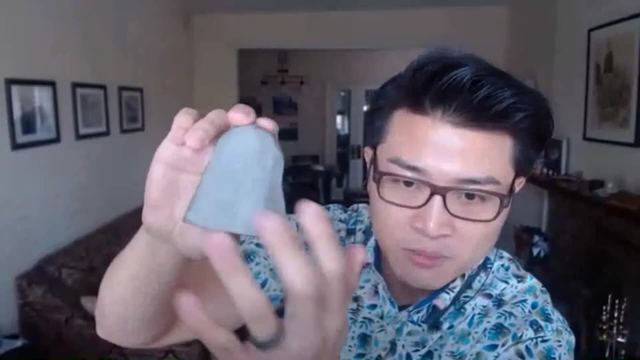 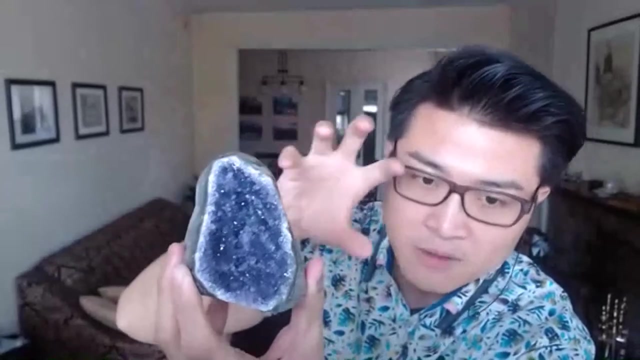 of purplish color, And so geologists think that the way this rocks are made in the natural form is that it used to be a piece of lava And there's some kind of heterogeneity And you can see here in the lava and you form this kind of liquid bubble. where the bubble 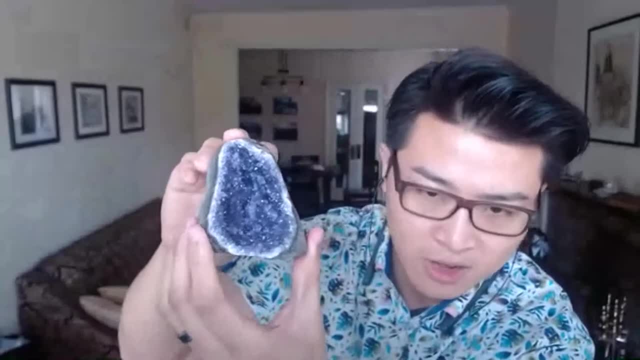 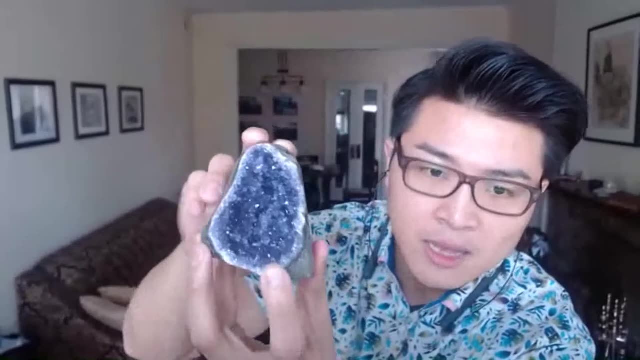 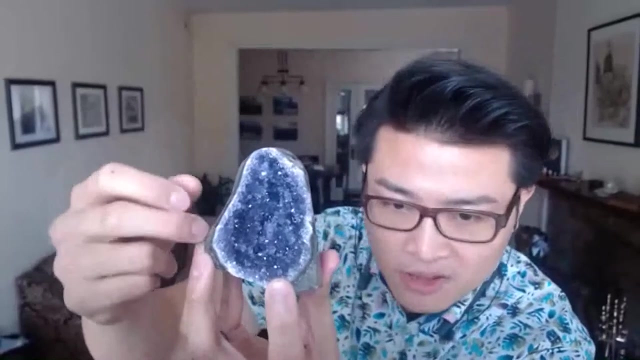 inside a molten glass liquid with silicon dioxide in there. As it cools down, then the crystal will then then the glass, or the silicon dioxide will start to solidify into solid. The process of it is very, very slow And because of that you have multiple what we 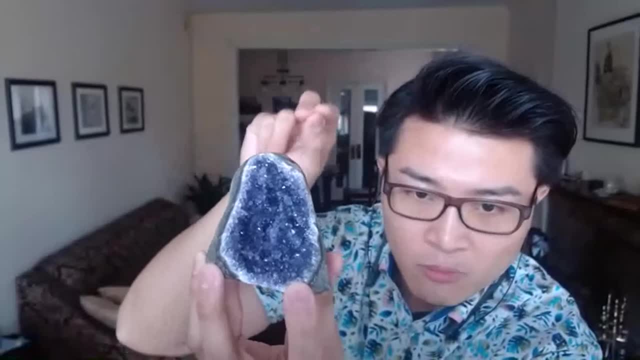 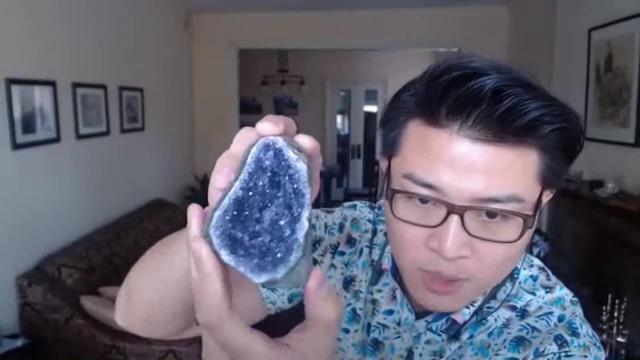 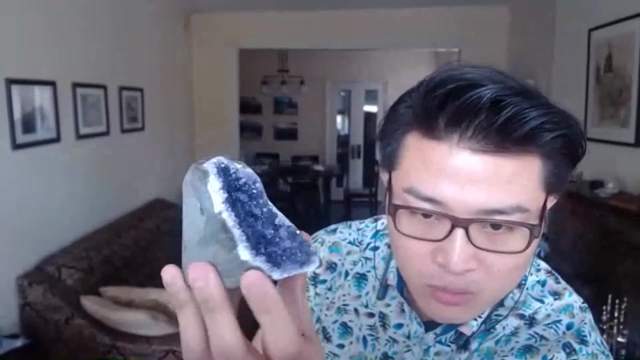 call new creation sites. So each of the crystal will grow from one location and another location, And then eventually they bonded to, they collide to each other, forming this what we call polycrystalline system. And so here I think that's like hundreds of them make each individual crystal have. 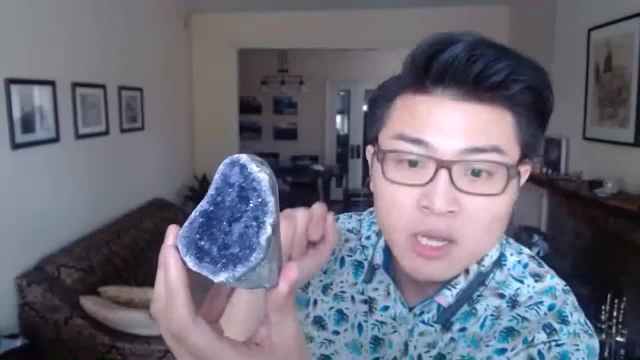 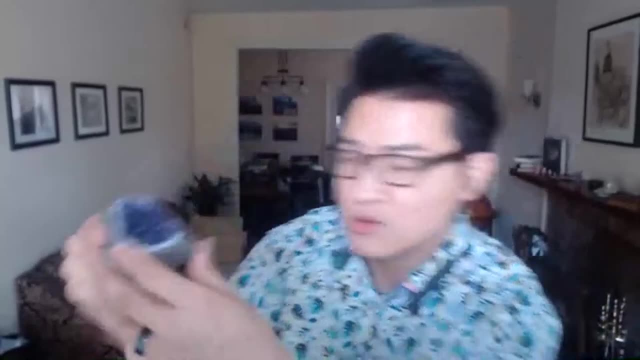 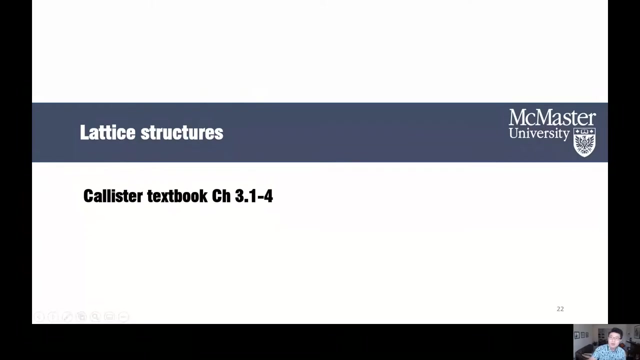 a different orientation, with same chemistry, same crystal structure, but just different orientation, making this really beautiful structure. I just want to show you that. Okay, So let's go back to the lecture. So in this lecture, we're going to be talking about 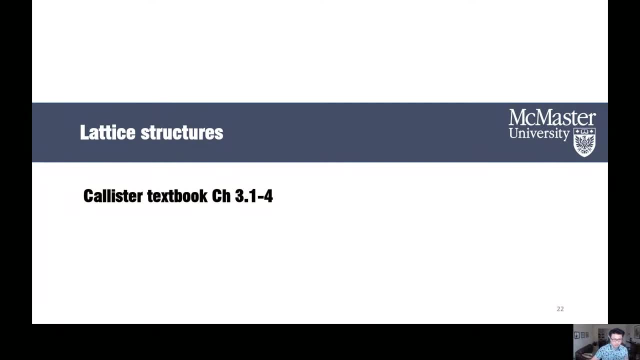 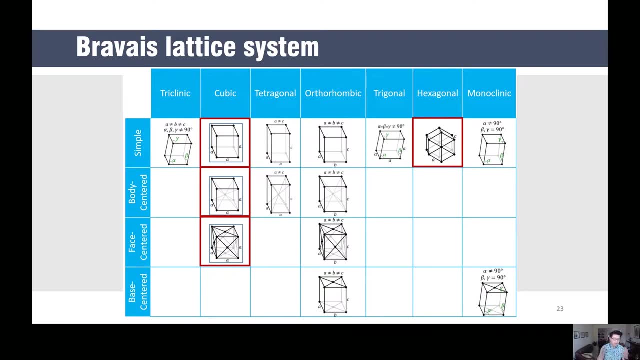 crystal structure, or we also call it lattice structures. So in this lecture we're going to be choosing a system where we call what lattice is. So earlier I showed you those beautiful crystal. Essentially they are atoms bonded together. And the last lecture: 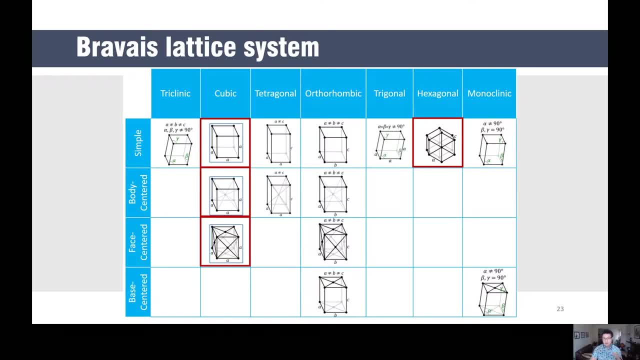 we talk about how, when you bond things together, they have different type of bond. They have atomic, ionic, covalent bonds, But we were talking about two atoms bonded together. Well, material made up of much more atoms in trillions. 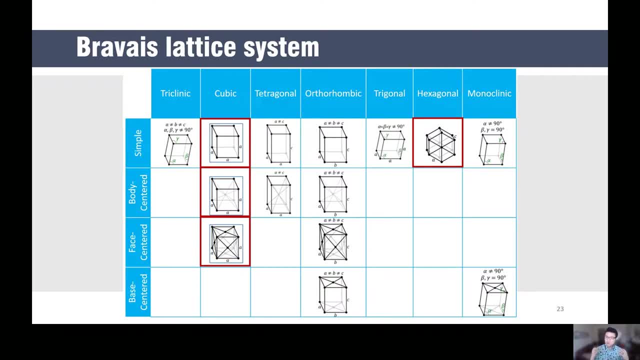 or even higher orders. And so how do atoms stack together? They are kind of like Lego blocks: One atom is one unit, and then two atoms bonded together, But then there could be another one, third, fourth and third, And then there could be another one third. 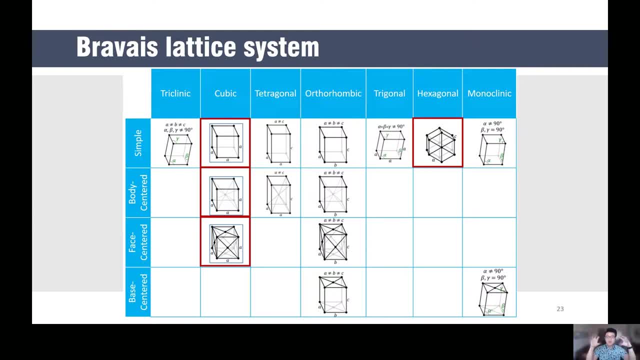 fourth and third, And then there could be another one third, fourth and third, And then there could be another one third, fourth, and then there could be another one third and third, And then it might look almost special. 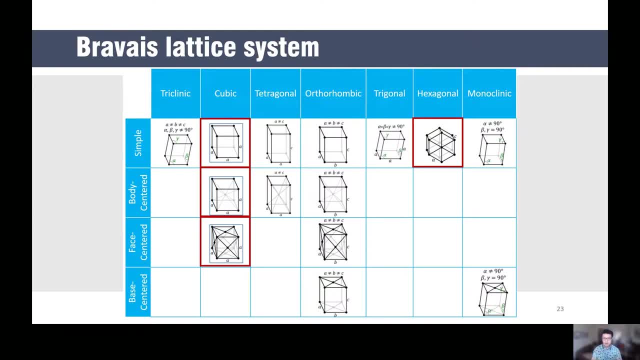 Physical dishes 활동 in zamano . And at the membrane of those atoms are caves, and we can call it geological structures, they actually deal with carbon electrons. They already join into that really big structure and then tissue again. And of course through the ​​ squatting in the relevant channels around them, 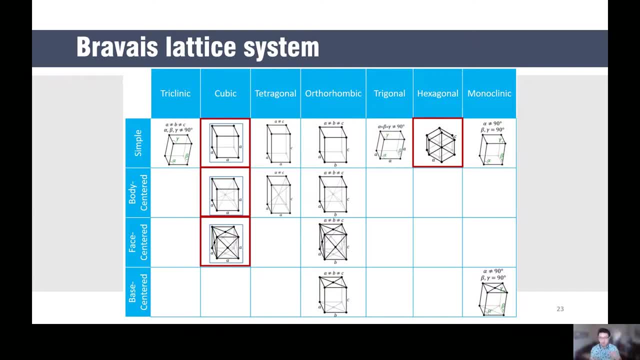 these glial cells that lead tohta want to Sonics, Then they're produced into everything other than the noodles all the way to it, And so I hope you can picture the latter all view, And we're talking about so many different sources. 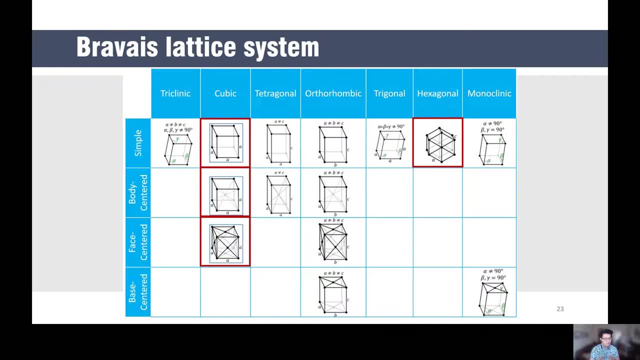 So I'm not going to give you the exact dates. it's the 1st or I'm just course. we're only going to touch on the surface of this beautiful and yet very in-depth study which are called crystallography, and in this study we're going to be talking about only the four different. 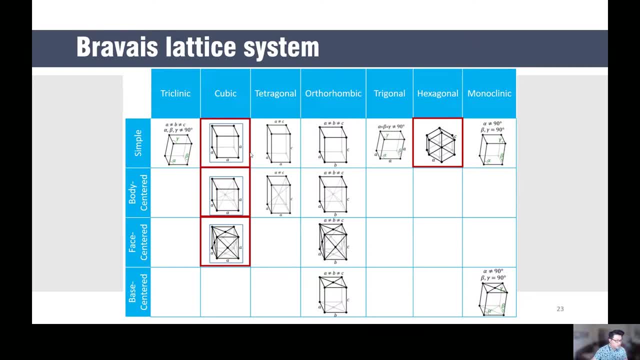 type of Bravais lava system. we're only going to be focusing on the crystal in the cubic system. so with simple cubic, body center, cubic. so body center cubic, face center cubic, and then we also briefly talk about hexagonal structure, leaving the other type of lava system for future years. so just want to let you know that this is a very deep topic and it 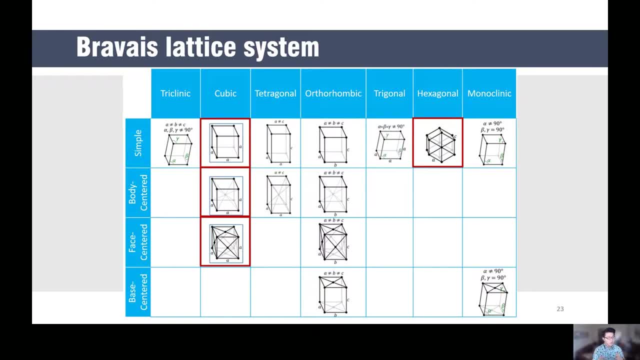 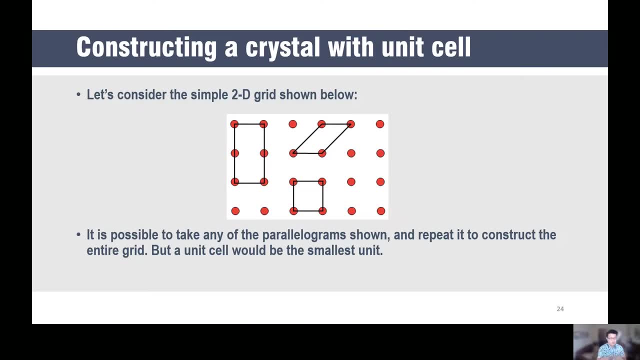 has a lot of fascinating physics and science coming out from that, but for now we're just going to be talking about the introduction of that concept. so what is a lattice and what is a unit cell? well, crystal is consists of many, many unit cells. so, for example, here i'm showing you a 2d image of a two, two-dimensional, simple square system. 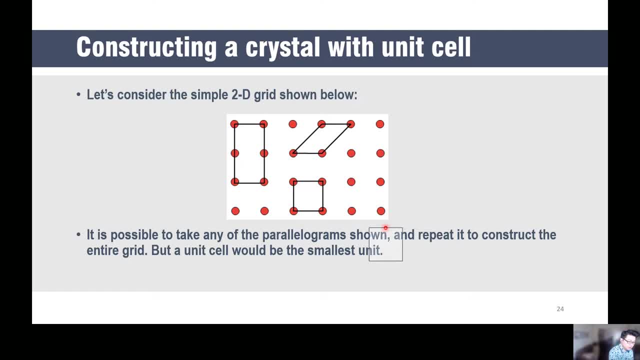 and we can define a unit cell to be a square. let's say then: here we have a square, and what is cool about this square is that if i just look at this particular square right here- so look at number one- i have a square with four quarter uh atom inside. this makes it one atoms, um, and so 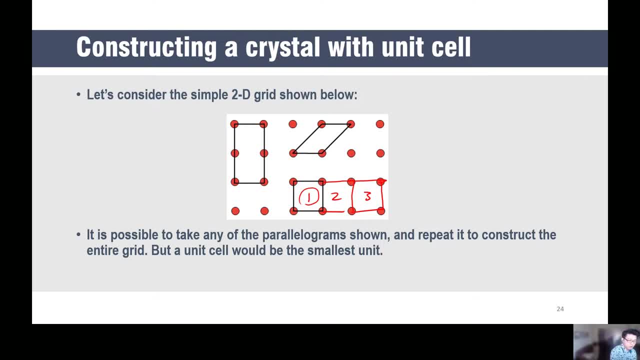 what is cool about this is if i look on the right hand side- let's say we call this the right hand side the x-axis and we call the um going upward is the y-axis- then we can find that if i just move my imagine you have a magnifying glass and move your magnifying glass to the right hand side. 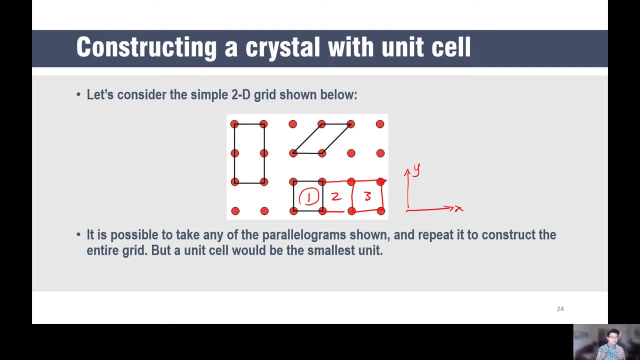 um, all of a sudden, i'm looking at the same thing. so this is called translational symmetry. and um, in the bravary lattice system, this 14 units, 14 type of lattice, all have translational symmetry in the three-dimensional world. and so here's a 2d system where we have a simple qubit. 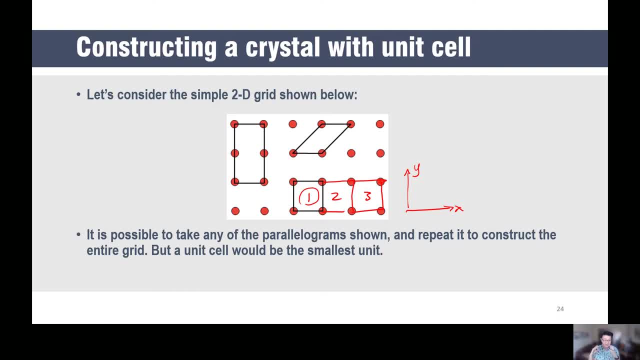 where we can translate onto the right-hand side and we just look at it and it looks identical, which is beautiful, because what it means is we can think of this one unit cell as a two-dimensional unit cell and we can simplify things, and i just look at the same thing for four units. 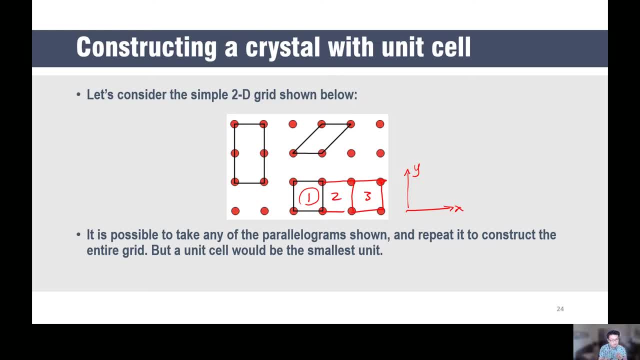 cell and we can just take that one unit cell and we can take that one unit cell as a building block. we don't need to think of the entirety. we can simplify things and just look at one unit cell, understand the unit cell, understand the property, and then we can just extravaganza from it. 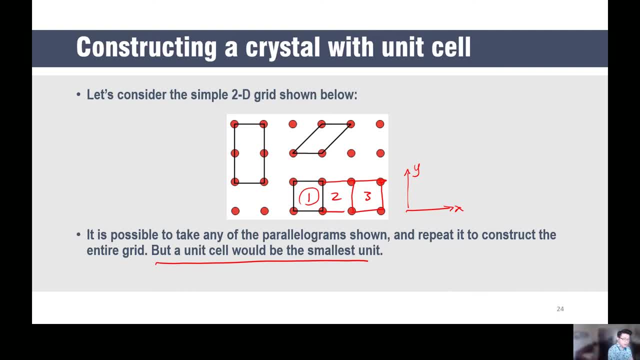 and so a unit cell would be the smallest unit inside this translational symmetry grid. in this case, it's x and y, and what is cool is it can translate in both x and y direction. so here, define a unit cell. usually, what we want to do is we want to make sure that the unit cells have the 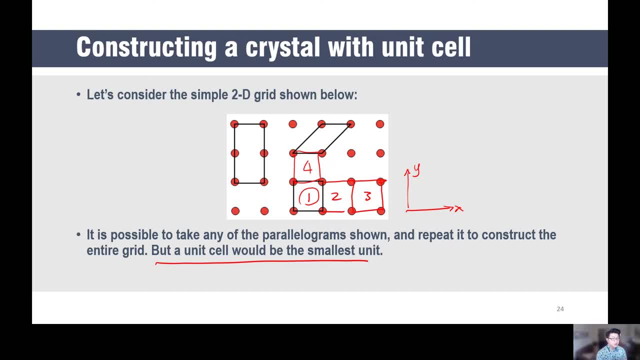 highest symmetry. So in this case the more appropriate unit cell would be a square. You can potentially define a rectangle, but in this particular case this rectangle is not the smallest unit possible, because the square would be. So that is a redundant system. 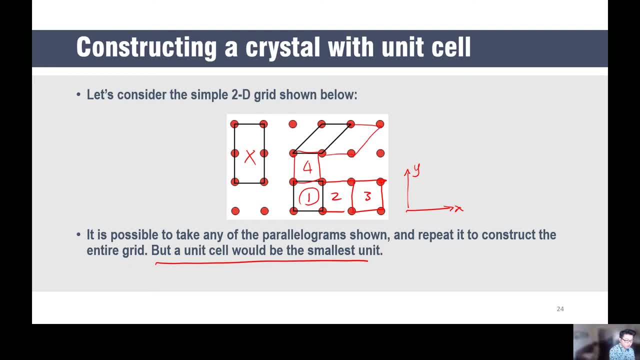 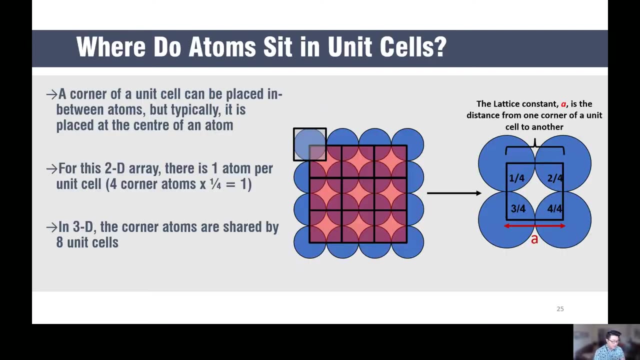 And then in terms of the diamond, although it's potentially possible to form that kind of unit cell, we tend to prefer to call unit cell that have a high symmetry, And so in this particular case we prefer a square system, And so you might ask: where do the atoms sit? I kind of hinted at. 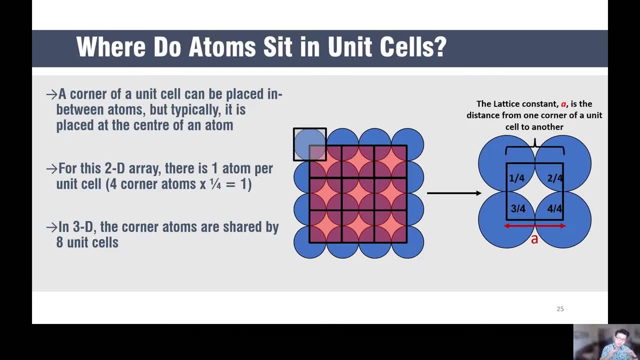 that already. So to give you an idea, the Larder system is a mathematical system to construct to understand how atoms are arranged together And each of those Larder points or nodes we call motors. Now I'm going to change the terms of the term, So we usually have a single atom in the 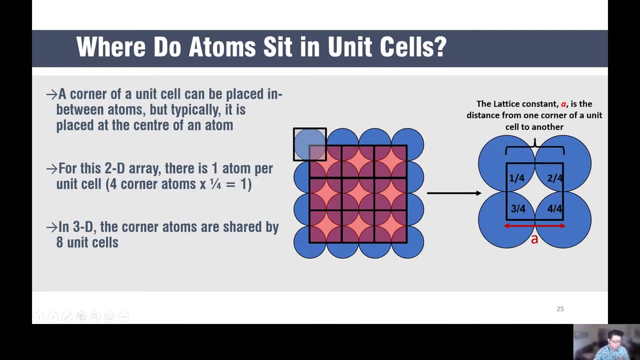 nomenclature. And then we have a single muscle in the nomenclature, a single block of the unit cell. So we usually have a single molecule in the nomenclature, And in that nomenclature we usually have a single mole, or at least a single molecule. So in the simplest case, 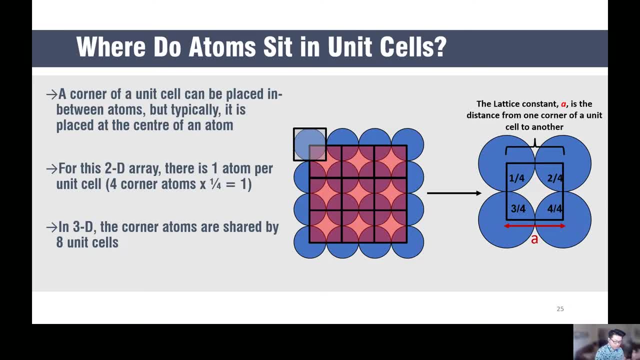 we'll have one atom inside this node and we call that motive. But it helps us to understand the nomenclature. So this distance, previously we call R0, which is the atomic separation In this particular case, R0 is actually equals to A. 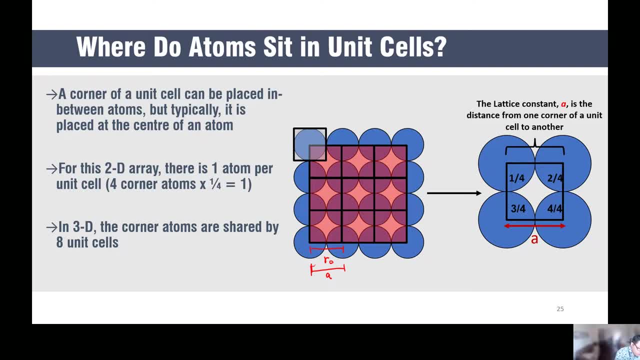 And so we have a simple square system. A is the lattice parameter. It describes the length or width of the lattice, not necessarily the atom, but the lattice, And so a crystal is created by a lattice grid plus a motive, and the motive could be an atom. 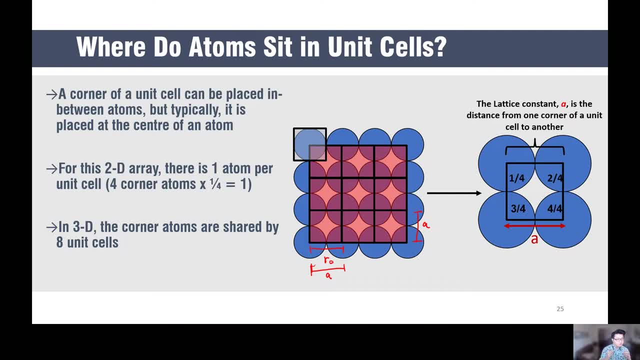 So in this case, you might ask: where does the atom sit? Well, it sits in the corner of this particular square unit cell. And so how many atoms are in there? Well, Well, if you look closely, each of these corner atoms, they're not all inside this grid. 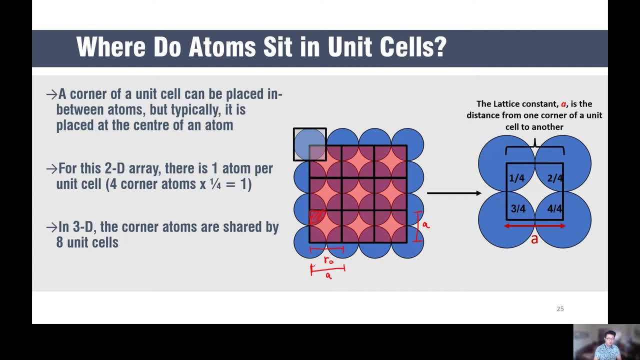 Only one-fourth of that atom are inside this grid. So and in one square we actually share four atoms, So four corner atoms each have one-fourth of an atom. So in total we have one atom for that particular unit, cell. 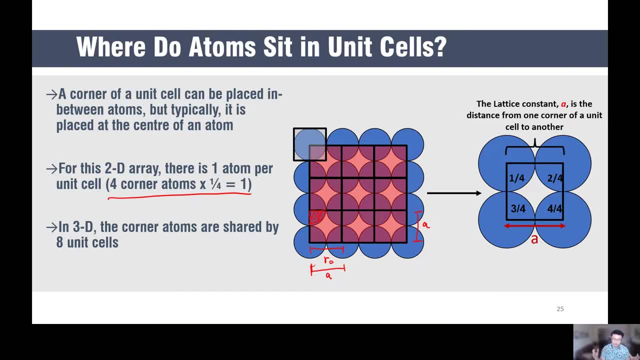 Now, soon you'll find out that atoms are made in 3D. They're stuck together in 3D network, not 2D. So a corner atom at a 3D unit cell will be one-eighth of a size. 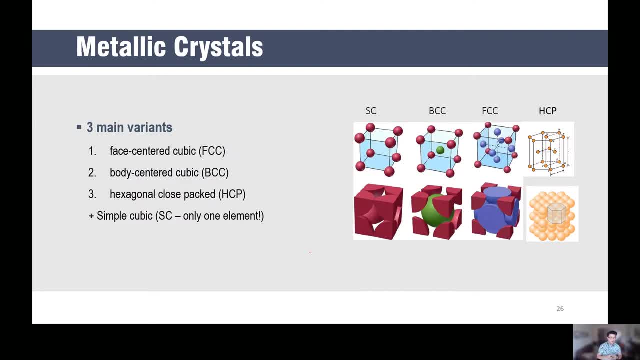 OK, So, like we said here, we're going to be talking about crystal system And we're going to simplify it ourselves, And we'll only talk about the metallic system, because metallic bonds are less directional And they're easier. They're easy to understand. 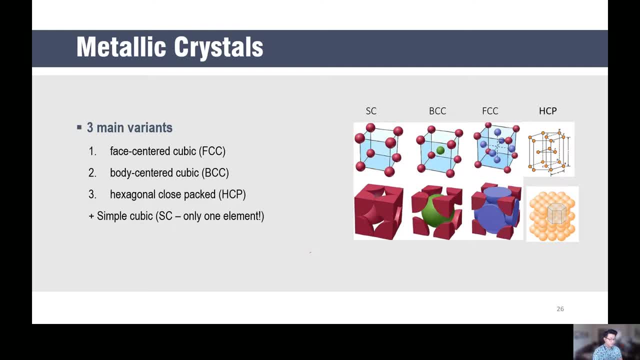 And so in metal there are many types of crystal structures, But the most common type are FCC, BCC and HCP. And then we also add one merges called a simple cubic. Simple cubic are very hard to find in nature. Materials tend to not like simple cubic. 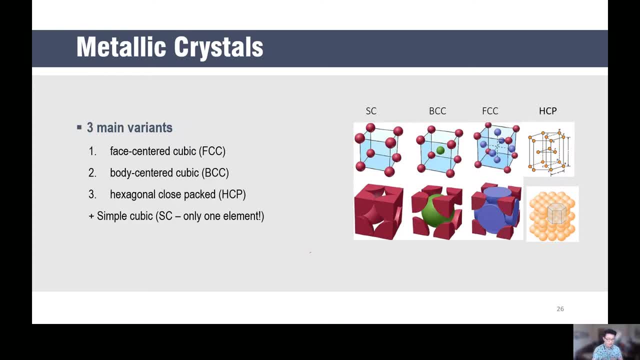 And you'll soon find out why, And it actually makes sense to you if you think about that. So let's start with a simple cubic cube. It's not a very structurally stable structure, And so it turns out there's a lot of gap inside this unit cell. that's making it not very cost-packed. 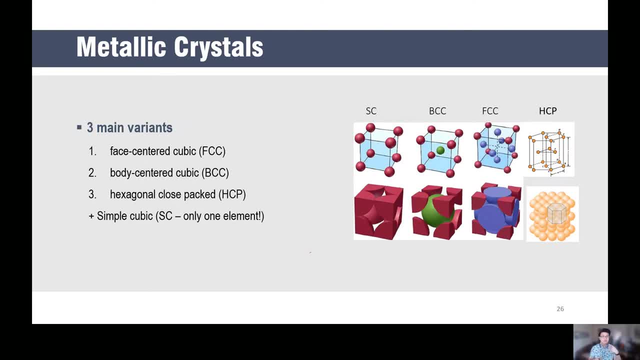 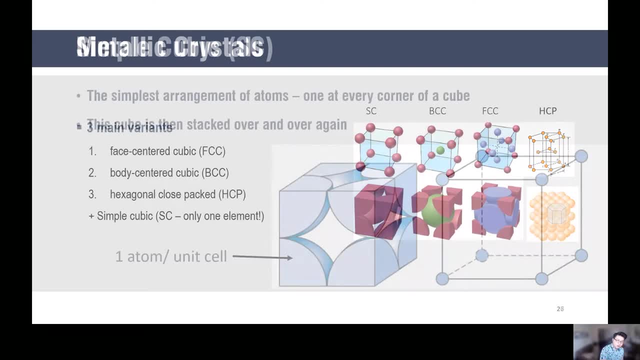 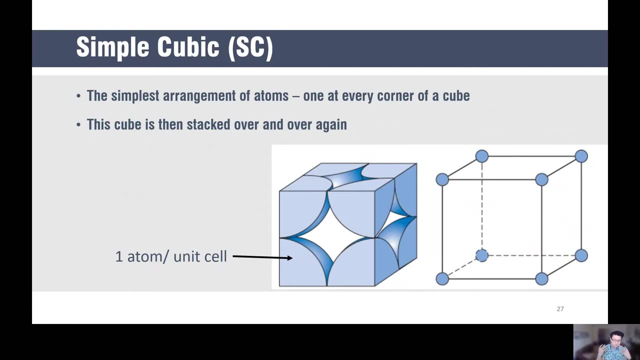 And cost-packed is something that's making it thermodynamically stable compared to a simple cubic structure. OK, So let's start off with the simplest concept of just understanding Bravais, lattice and understanding a unit cell, And by doing so we can go into some more realistic material. 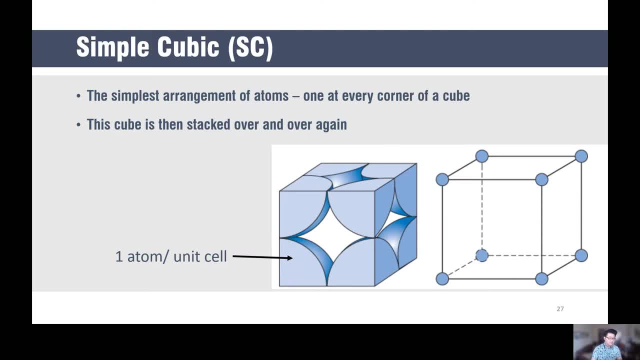 So let's start with this. OK, So let's start with simple cubic. Simple cubic is the simplest arrangement of atoms in 3D, which each corner have one-eighth of an atom. So this corner, for example, this is one-eighth of an atom. 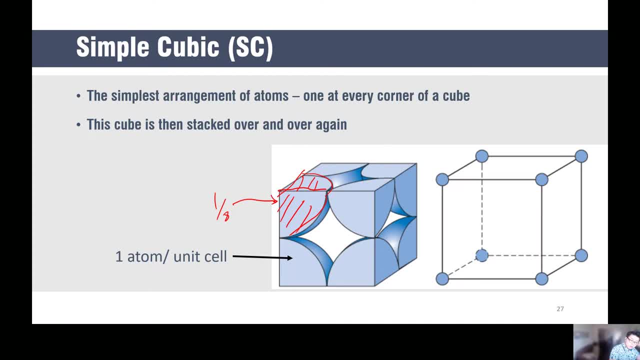 And so to draw a unit cell, there's two ways to draw that. The left-hand side diagram is actually the more realistic way of drawing things, Where an atom, represented by this ball and really is actually an electron cloud with that particular radius And in this particular case the X, Y and Z direction, all have a parameter of A. 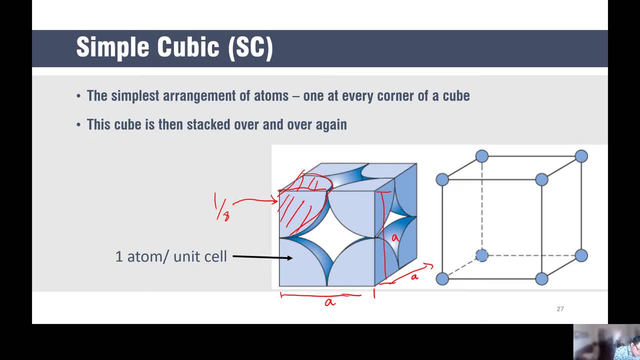 A is the largest parameter, In this particular case the atomic radius. Atomic radius is R, is half of the lattice parameter. So here we have also A here. So that's the atomic radius. So with that said, how many atoms are there? 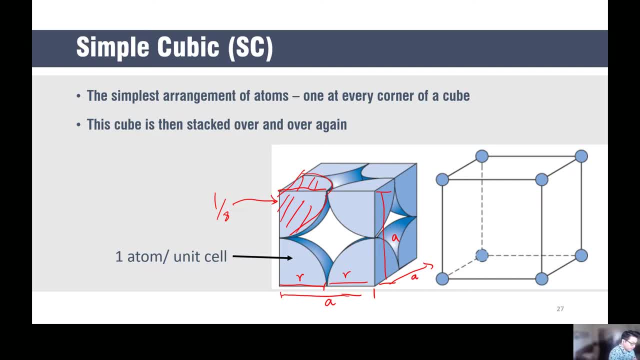 Well, each of them, we have eight corners Atom And each one is one-eighth. What that means is that we have eight times one-eighth of an atom, which is equal to one atom per unit cell. This is the simplest you can get. 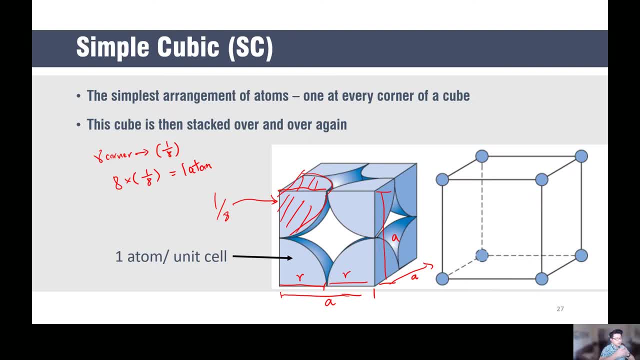 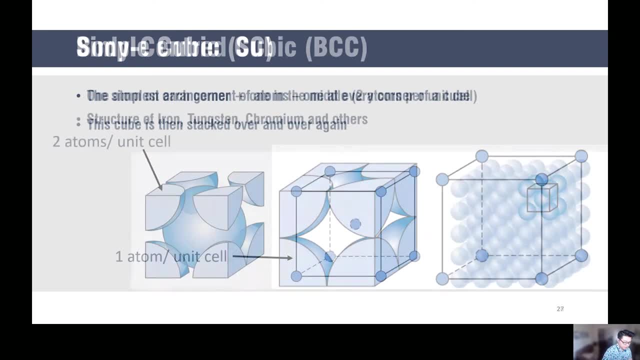 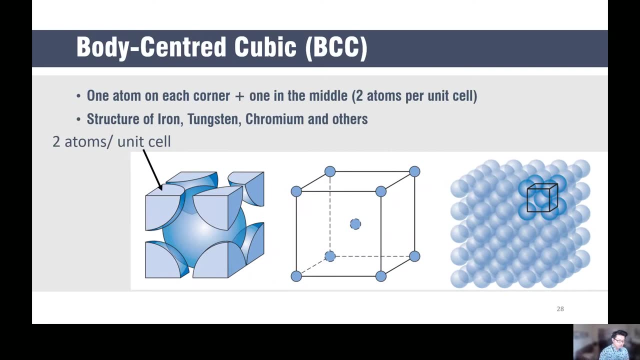 And you can think that this cube can just stack in the X, Y and Z direction, Kind of like a Lego block making a crystal structure. The next one is called the body centric cubic And in this particular case this is the realistic system where structure of iron, tungsten, cobalt and other type of metal- usually ferrous materials- tend to have this kind of BCC structures. 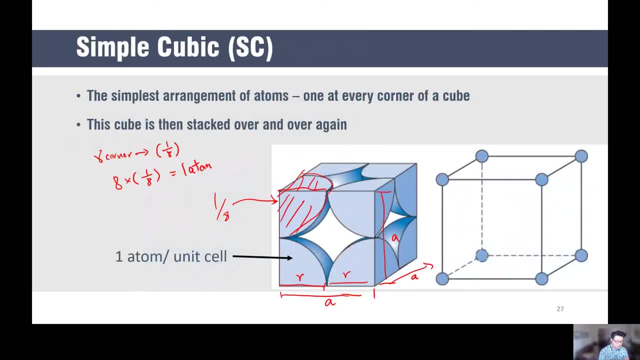 So, if you compare to the previous one, which each of the corner have one-eighth of an atom, Now what we did is we're going to stack one more atom inside this cubic And we're going to stack it inside its body, And that's why it's called body centric cubic. 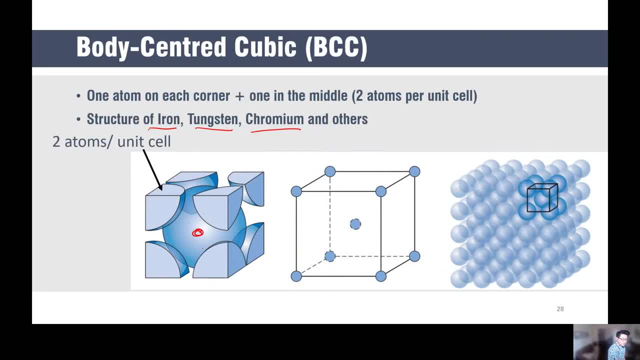 And so there's this one extra atom here, This one extra atom, And so this is one atom. And then, so how many atoms are inside the unit cell? We have plus eight times one-eighth, which is equal to two. OK, so these are the corner atoms. 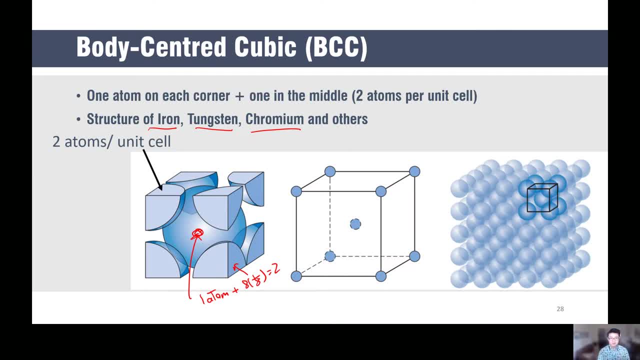 Right. So a body centric cubic consists of one body centric atom plus eight, one-eighth of a corner atoms. OK, And so the same thing. we will draw this kind of structure, And now A is representing the new lattice constant. 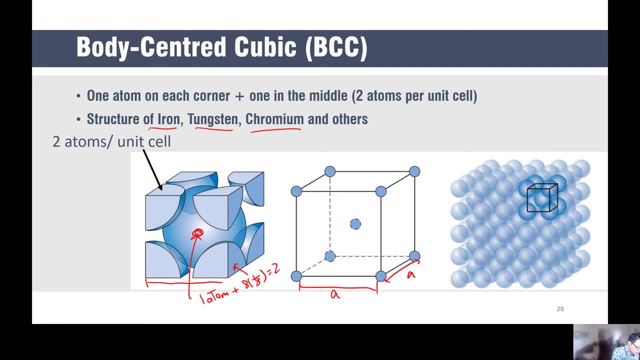 And you can imagine that this actually is no longer out. There's no longer two out A. This is no longer two out Because this is out, This is out And there's a gap there, So A is actually bigger than two out. 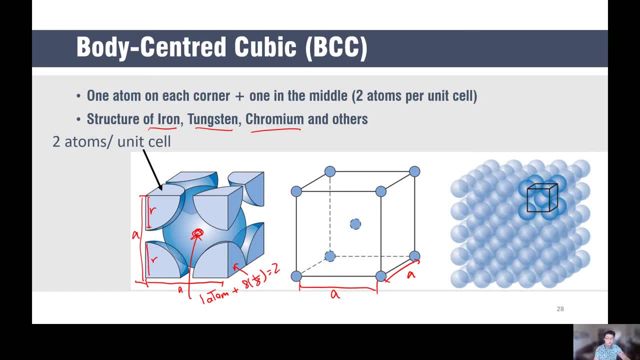 And soon you will find out that this is very important because this helps us to calculate what's the ratio between the atomic radius and the lattice constant And we can basically can get an idea of how packed are these atoms in comparison to a fully dense structure. 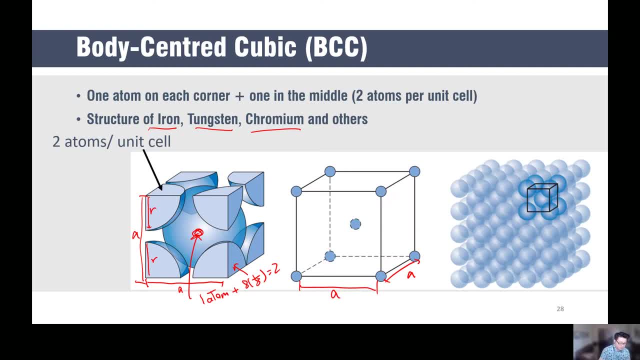 Right. So by doing that we can then calculate what is the density. And so here we can also see that, OK, well, this is one unit cell, and then this is another unit cell, and so forth, so on and so forth. 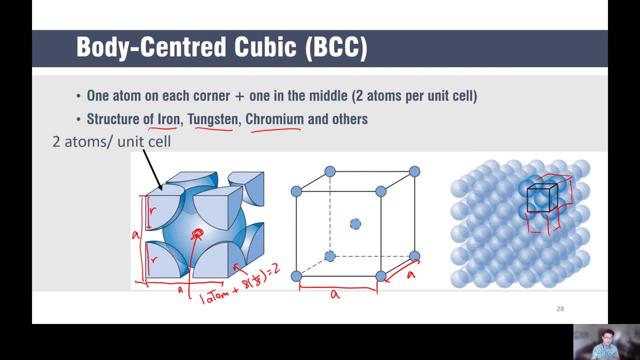 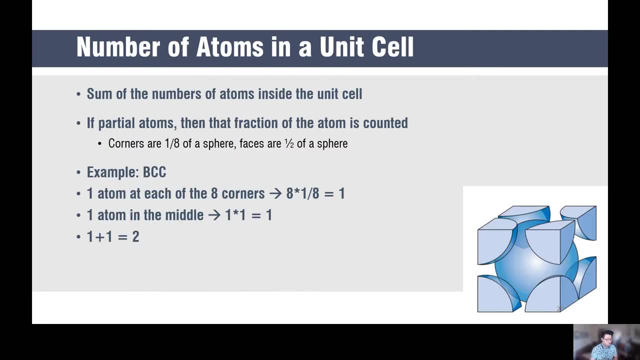 And so you can create a structure by stacking these unit cell together like a block. So it's just a summary of what we said. BCC: we have one eighth of an atom inside each corner, plus one atom in the center, creating two atoms per unit cell. 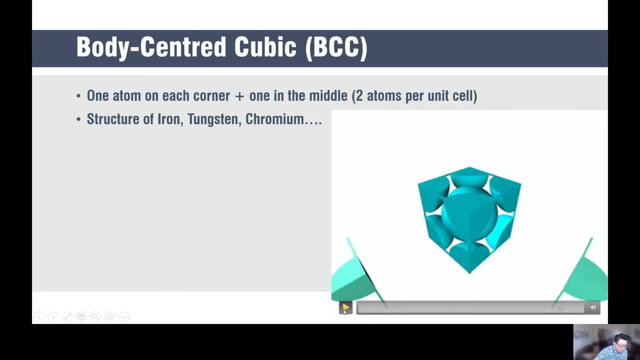 Now here I want to show you a video of how a BCC structure looks like For those that maybe need help with the corner atoms, how it actually is one eighth. So let's see the column. So this is a BCC. 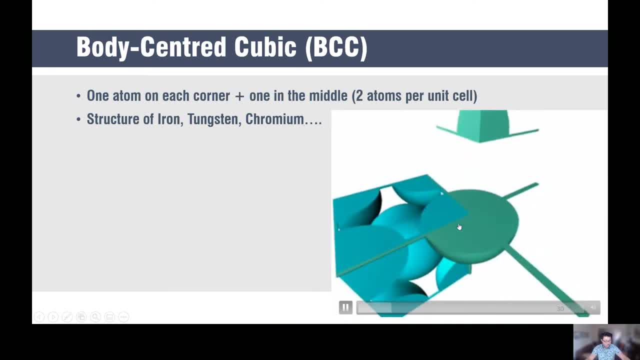 One corner involves one, two, three, four, six, five, six, seven, eight, Eight pieces of corner create one atom, And so BCC corner involves one eighth of an atom. OK, Hopefully that's clarified why BCC has two atoms inside each unit cell. 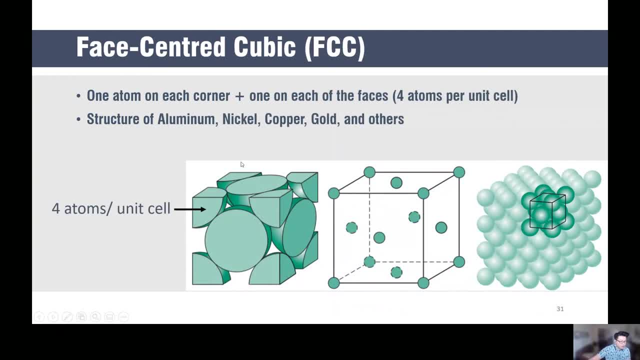 Finally, in the next one, we have what we call a phase, centric, cubic, And the reason we call it phase is, instead of stacking one atom into the middle, we now stack the atom onto the phase of each of those lattice, And so we now have a unit where this is A: 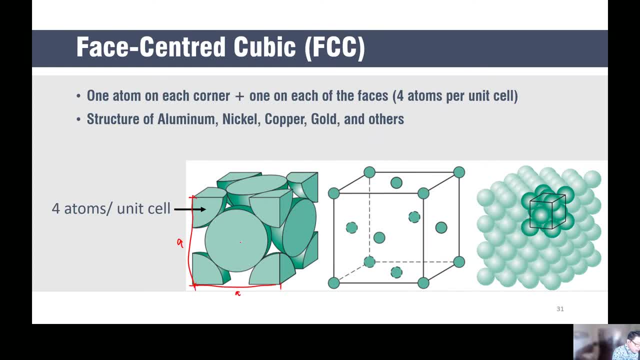 This is A And we have one. Well, we have four, One, two, three, four, five, six, Six extra atoms that are half. You think about that? So these are half atoms. Sorry, let me just erase that. 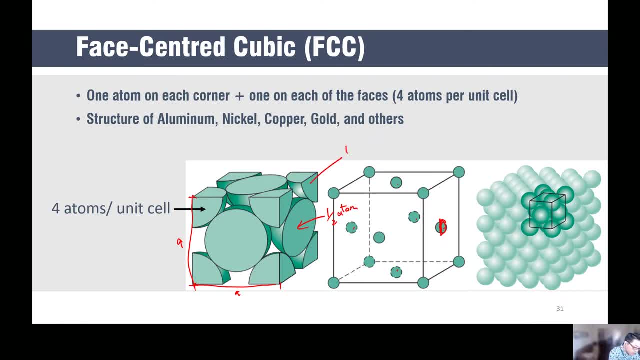 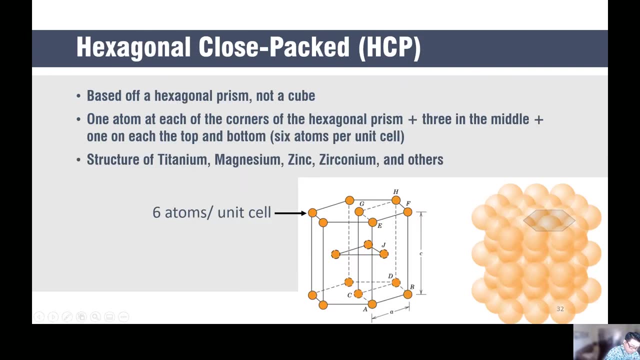 These are half atoms. Now these are one eighth of an atom. And so how many atoms? And so how many atoms are inside? Well, we have how many phases? One, two, three, four, five, six. So we have six phases. 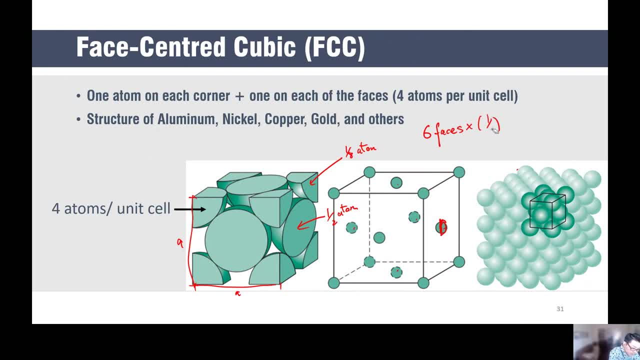 Times, one half, Plus we have eight corner Times, one eighth. So this is one atom, This is three atom, which gives me four atom per unit cell And turns out FCC is a very common material that are being used in many structures. 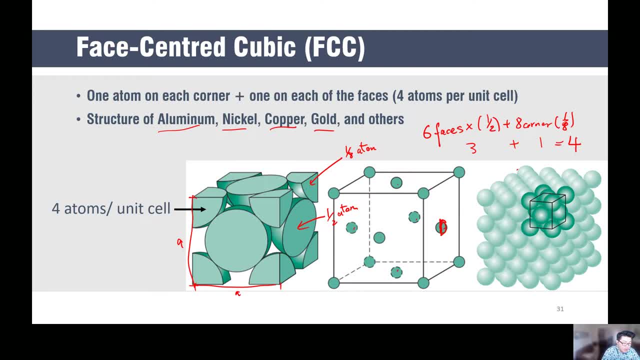 Aluminum, nickel, gold and so forth, And FCC structure is a very interesting structure because soon we'll find out from the next video that turns out FCC have one of the highest packing factor, making it one of the densest possible structure, And so it makes sense why dense materials such as copper and gold- very heavy metal- tend to have FCC structure as well. 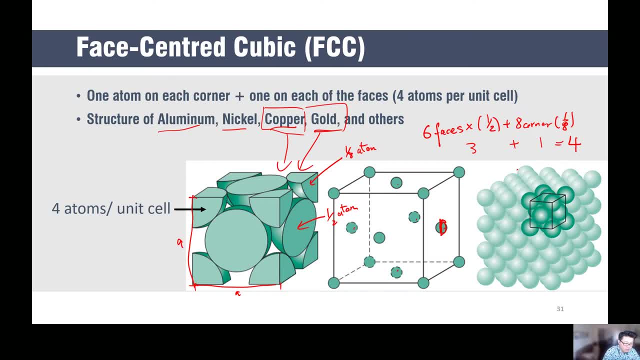 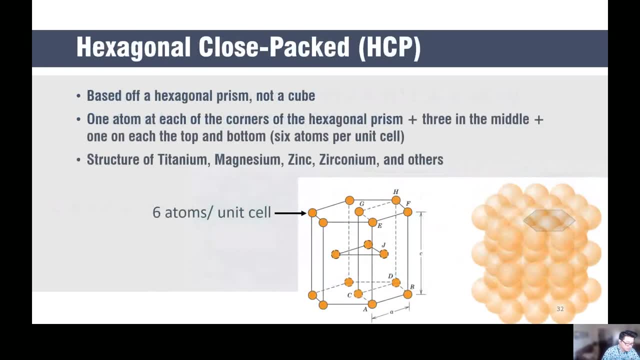 And turns out many element. when they are at the ground state, meaning at the lowest temperature, they prefer to be in this particular cost pack structure. The next one is called the HCP, which is the hexagonal close pack structure. So it's actually very similar to FCC if we dissect it. 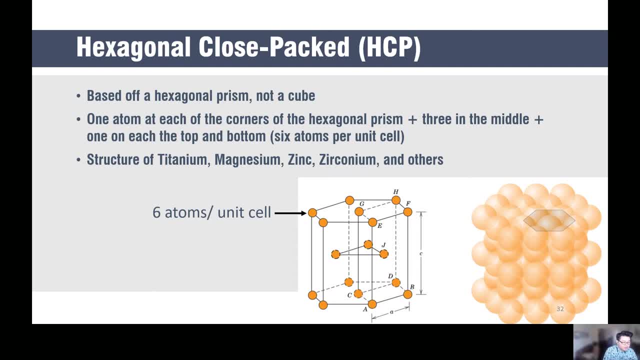 But right now, looking at this hexagonal close pack is referring to a structure where there is a basal plane, Where these atoms stack to each other almost like a hexagon or prism structure. And so here you can see that this is hexagon: no structure constructed of six different triangles all put together. 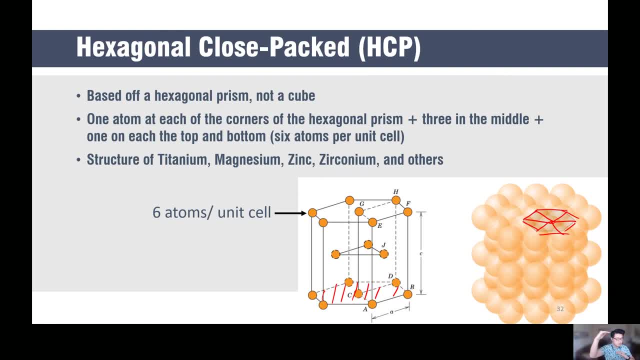 And they just stack in this AB, AB, AB stacking This particular crystal structure is also very interesting. Titanium, magnesium, zinc and zirconium are made of this structure. Magnesium is a very interesting alloy, actually Very interesting, Very interesting metal. 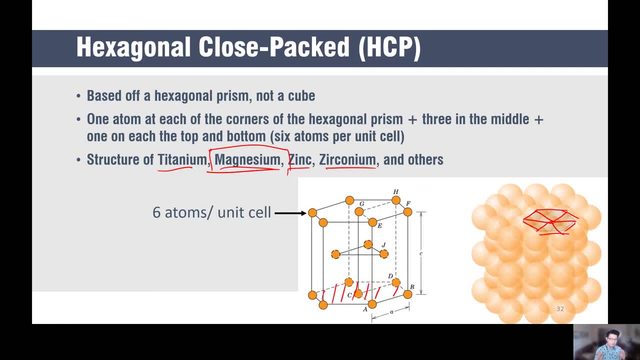 And the reason they are interesting is that magnesium is extremely lightweight but also very, very strong with a drawback, So a sink is very brittle And turns out that HCP is a structure where, because it has this close packed plane and then a separation, 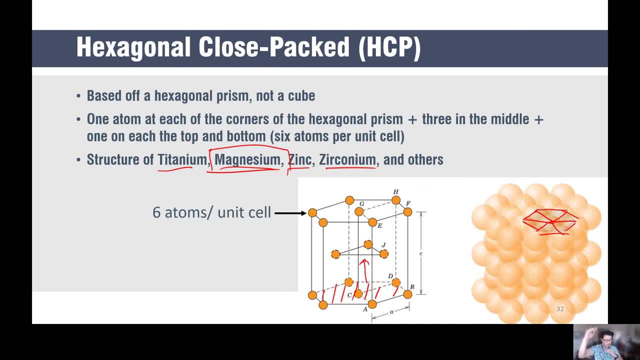 And that separation from plane to plane, a stacking. depending on that separation you have very different mechanical property. And HCP metal tends to be relatively brittle. Brittle, meaning that it requires a lot of force but not necessarily a lot of deformation to break that material.